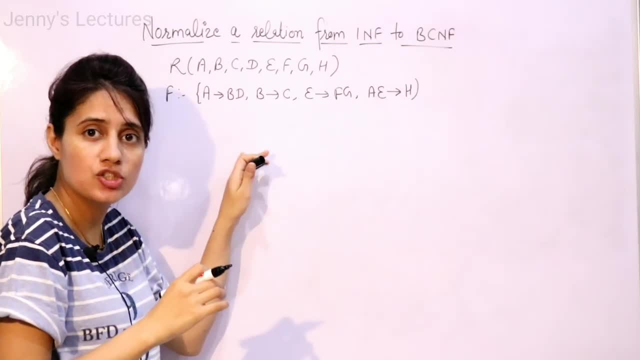 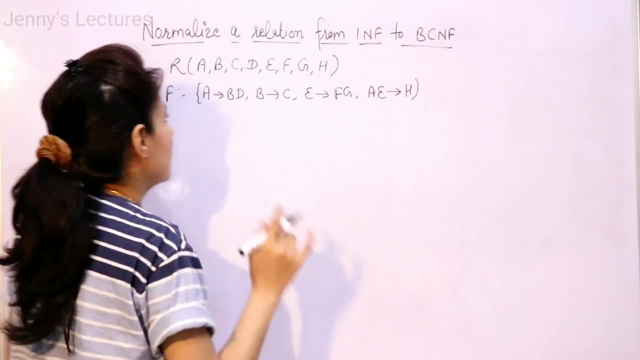 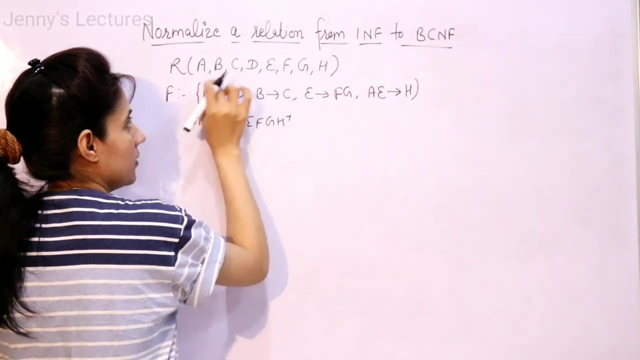 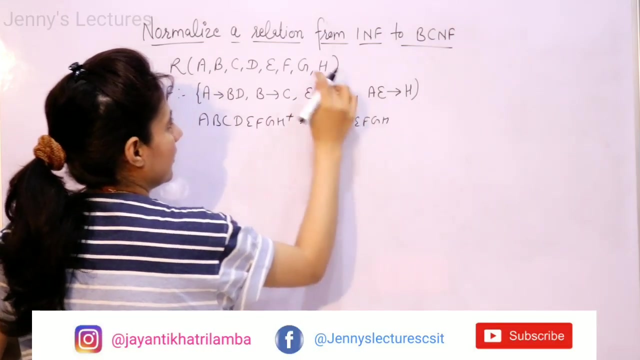 discussed how to find out candidate keys from a given relation in my previous videos. I will provide you the link of the complete DBMS playlist in the description box. you can check out there right. So now, take all the attributes of the relation and find out the closer. obviously it will find out all the attributes right Now. try. 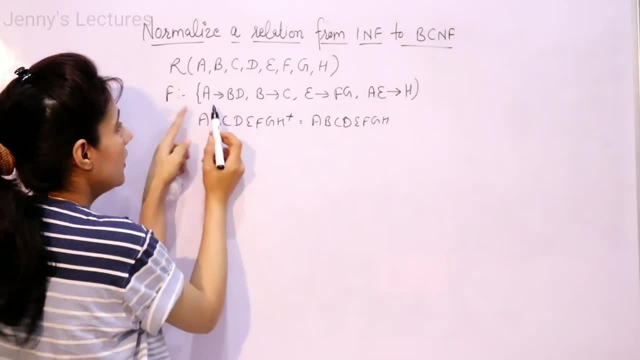 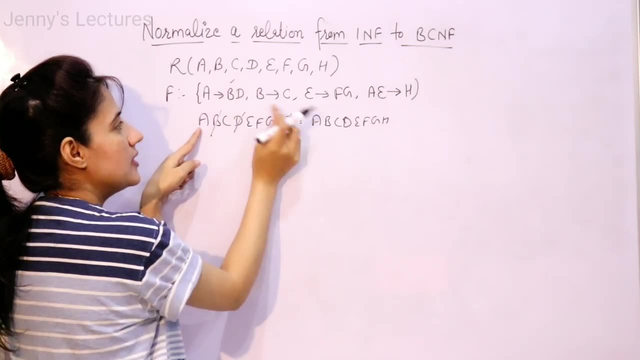 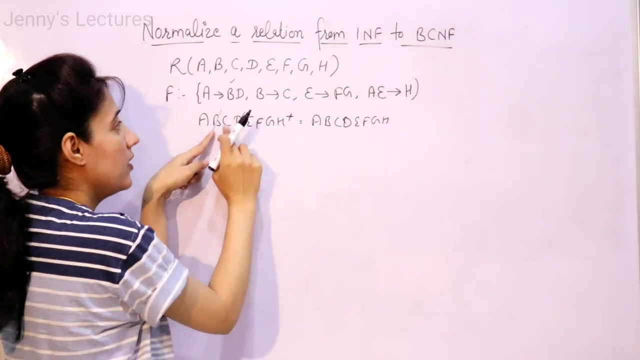 to discard the attributes using functional dependencies: right, A can drive B, D, so if you have A, I can discard B and D. right, See B can drive C means if you have B, you can drive C. Now, obviously, if you have A, I can drive B right, and if I have B, then I can drive C, so I can discard C. 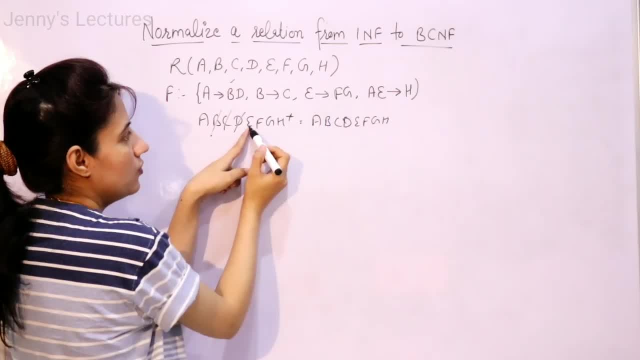 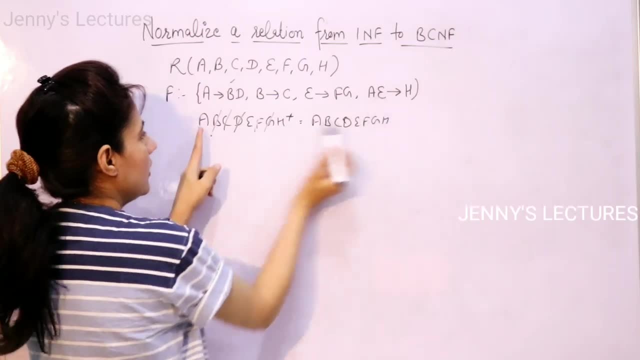 as well. Using E, I can drive E and F. so if you have E, you can discard F and G. sorry, F and G right Now. if you have A and E, A and E- so you can derive H, so you can discard H, because I have. 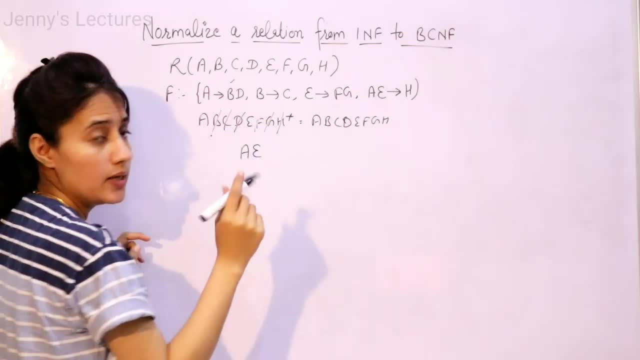 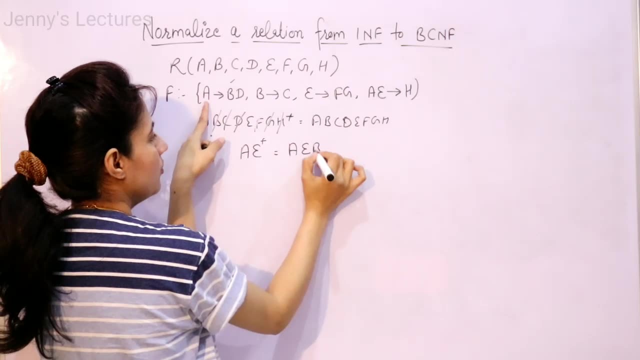 A and E. so the remaining attributes are only A and E. Find out the closer. C- Using A, I can drive A. E. definitely. Using A, I can drive B, D. Using B, I can speak. C. Using E, I can drive F, G and I can. 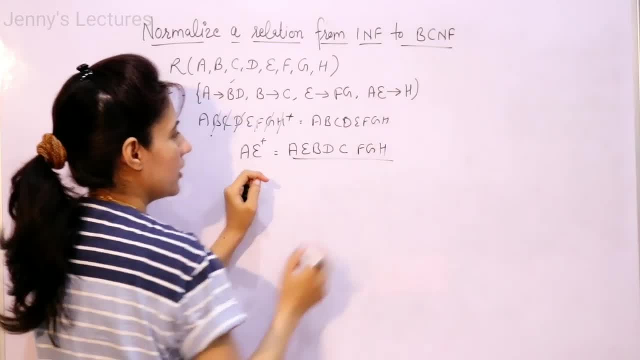 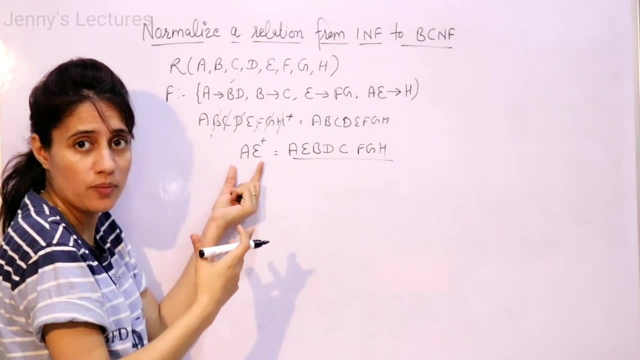 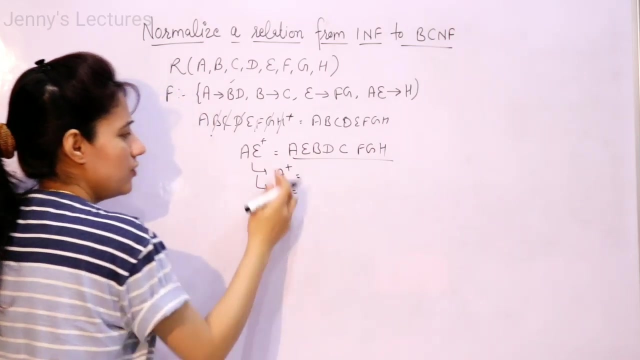 g and i can drive h, all the attributes i can drive. so a is what you can say, it is a super key. we cannot discard any more elements, any more attributes from here. so this is super key. now proper subset is a and e. obviously no proper subset would be super key, because 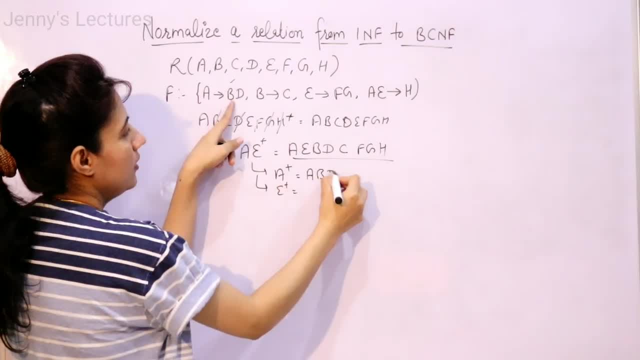 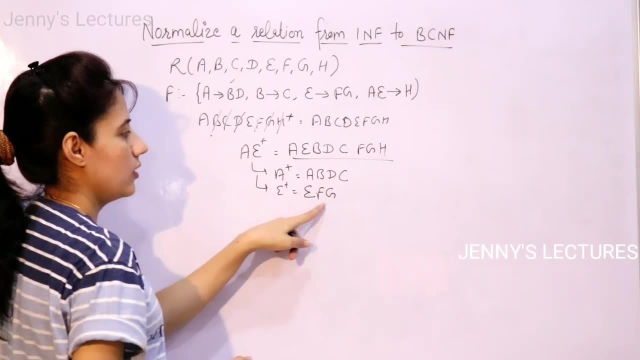 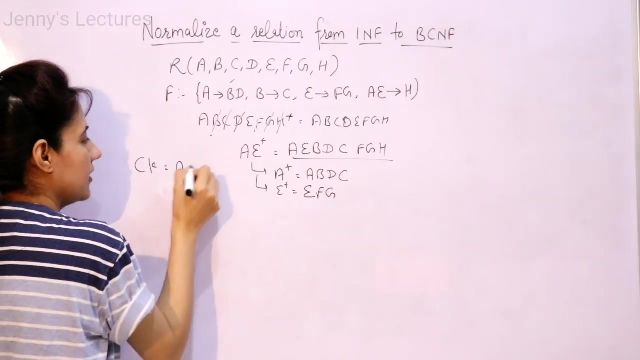 a closer would only contain a, then b, d, then we can drive c right. not all the attribute e closer can contain e, f and g only right. so no, this is neither this is super key or no, this is super key. so that is why we can say that a- e is our candidate key right now. 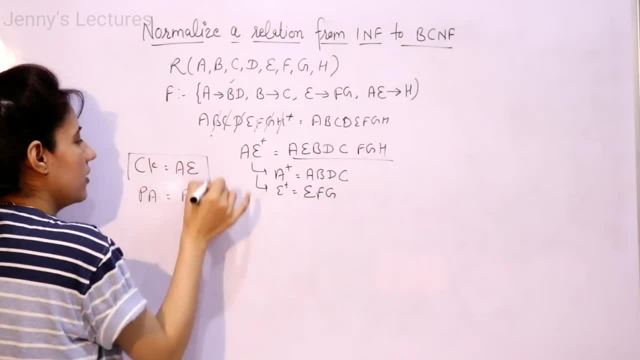 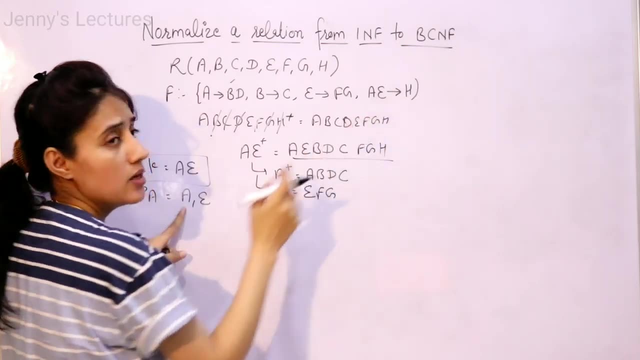 prime attributes are a and e. fine, find out more candidate keys are available or not. if prime attributes are available on the right hand side of any functional dependencies means there are still more candidate keys, but a and e are not on the right hand side, so there is only one candidate key. that 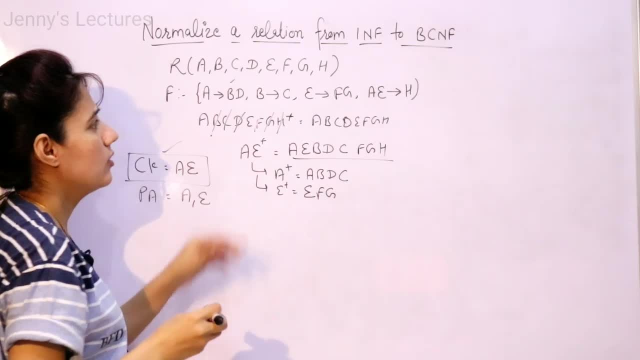 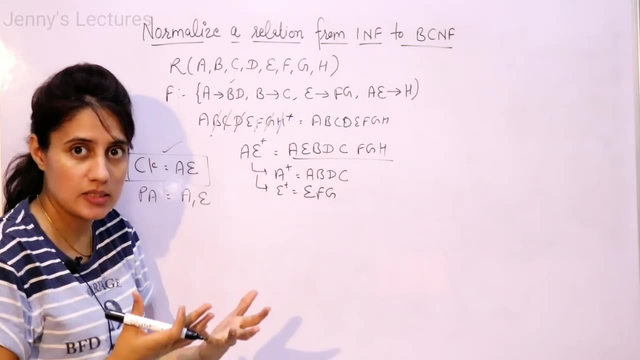 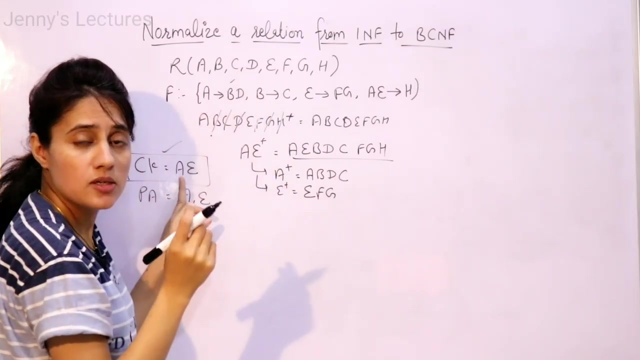 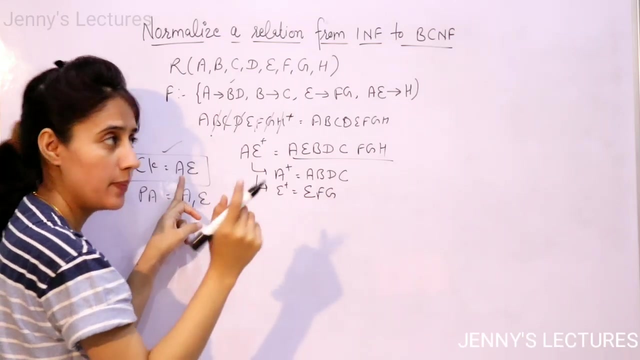 is a fine. now find out which functional dependency is creating problem. means which functional dependency is partial dependency. right, see, a can drive b d. partial dependency means the proper subset of this candidate key drives non prime attribute. then that is partial dependency. a is partial subset and b d. yeah, this is non prime attribute because 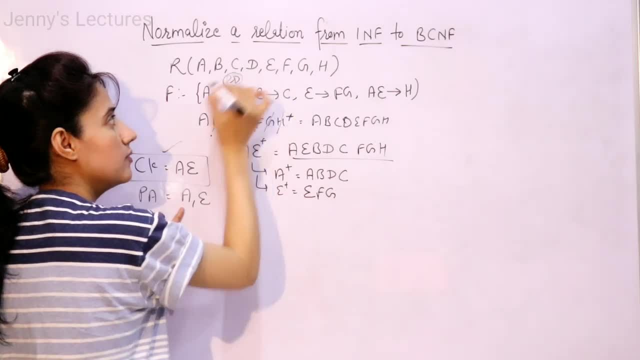 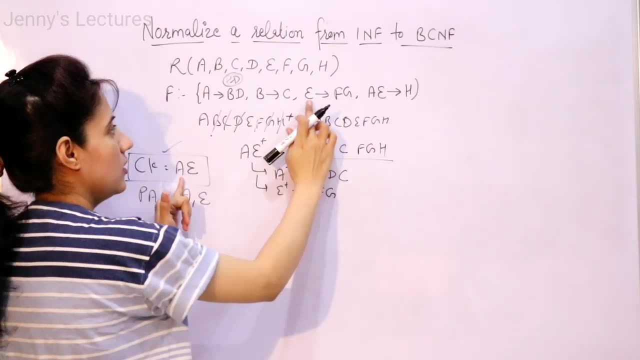 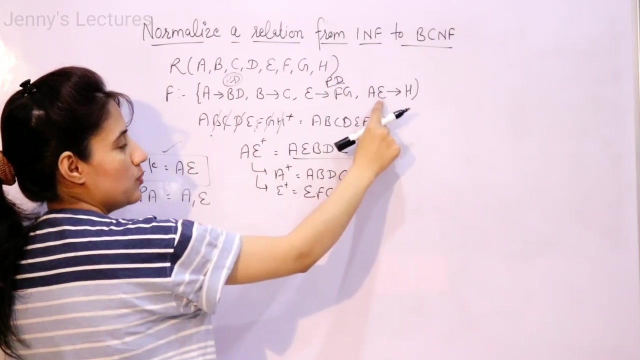 prime attributes are only a and e, so this is partial dependency. right s, b, proper subset of this one. no, so obviously this cannot be a partial dependency. e is proper subset of this one. yes, f, g are non prime attribute. yes, so this is partial dependency. a is proper. 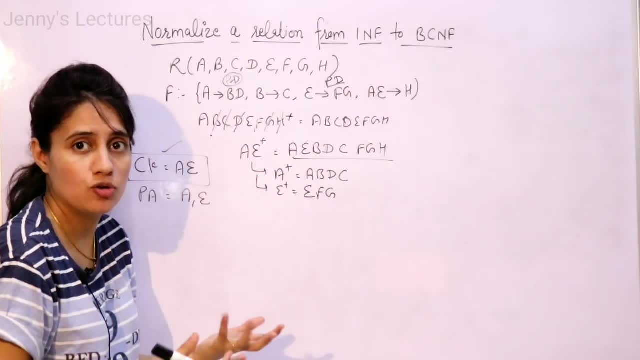 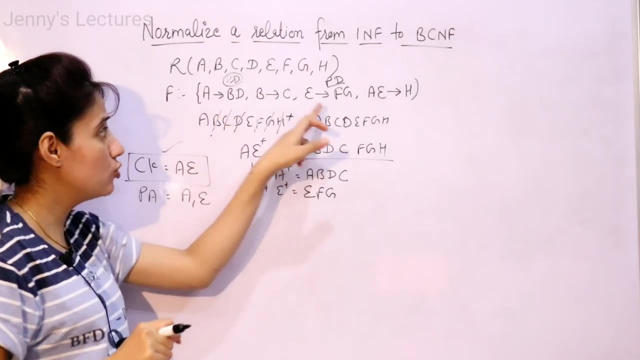 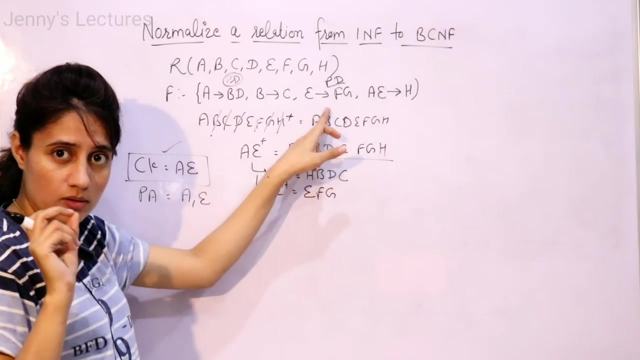 subset of candidate key no a. e is itself a candidate key or you can say super key. so this is not partial dependency, means these, these two functional dependencies are creating problem because of these two. this relation is not only in second normal form, it is in first normal form. now we have identified the dependencies. 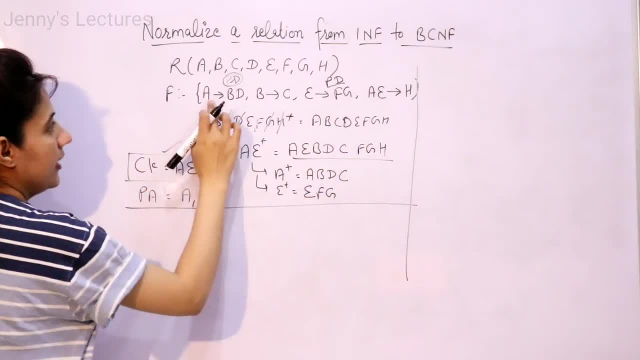 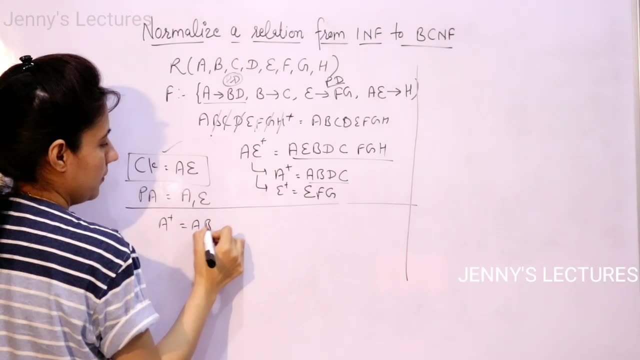 which are creating problem. so next step is what? take out this one, this functional dependency, and find out a closer. a closer would be this one: a, b, c, d, right. using these, i will find out. now, put all these attribute is in one relation: right. find out e. close, a be this one: a, b, c. 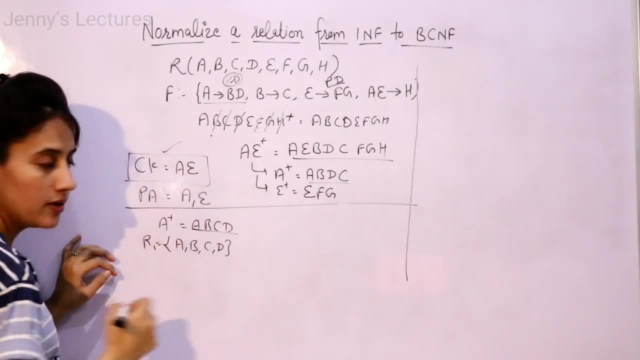 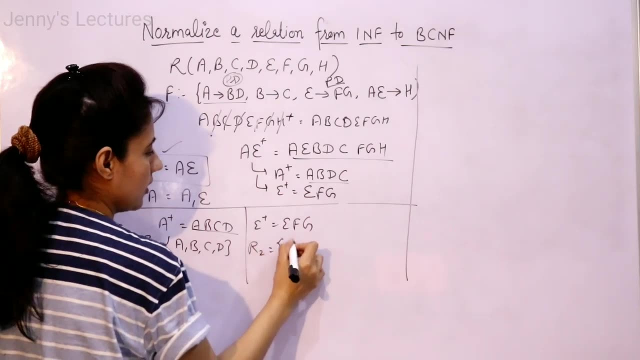 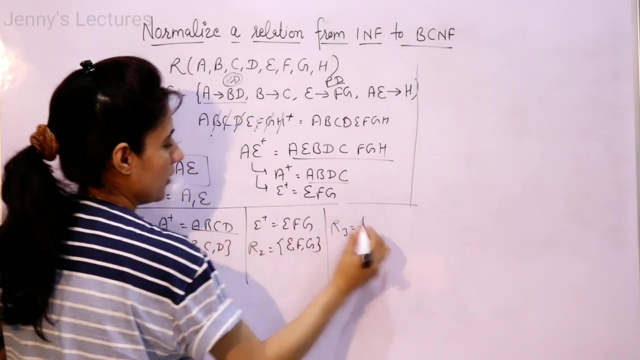 d right now. put all these attribute is in one relation right. find out e close, a is normal at 0.1.. closer e, closer would be e, f, g. put all these attributes in another relation right. and put all the remaining attributes in a third relation. remaining attribute is h only right. but we cannot. 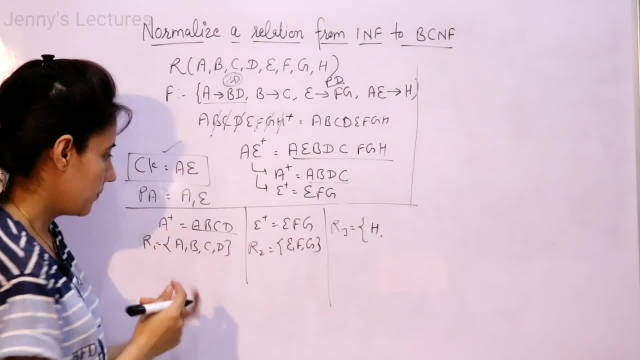 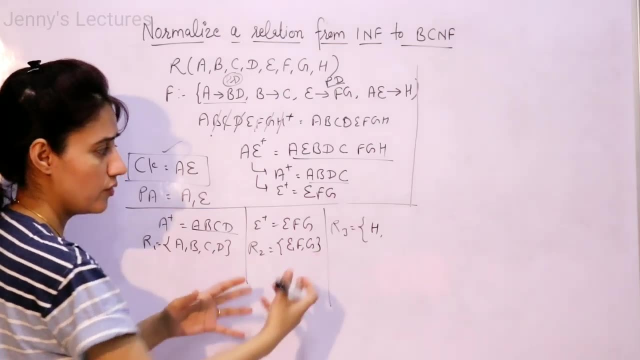 put only one attribute in this. so now what you have to do? see, now there should be something common, right, because in this and this there is no common, in this and this also no common. so when you will join, there should be something common, big to to be a lossless joint decomposition, right? if 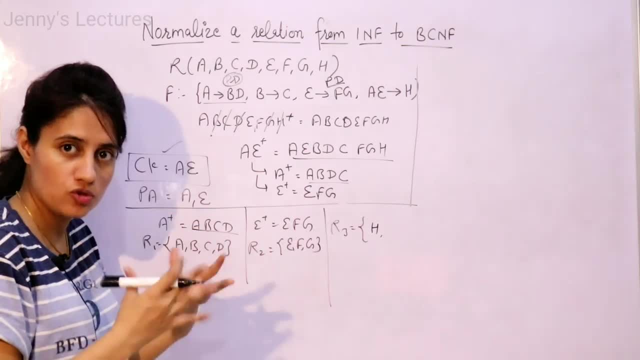 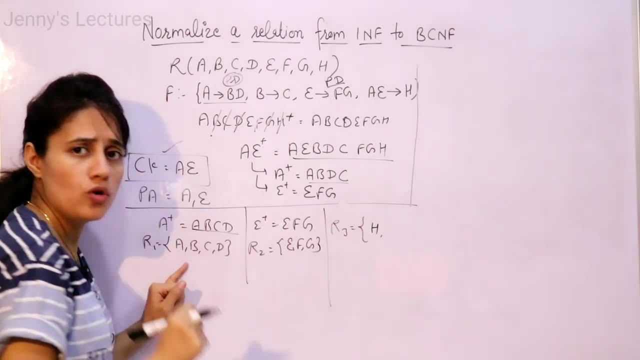 nothing is common between the relation, then this is lossy joint decomposition, right, and we want lossless joint decomposition and dependency preserving. so if we join this one in this one. so what should we put common here? see, the common attribute should be super key. or you can say: 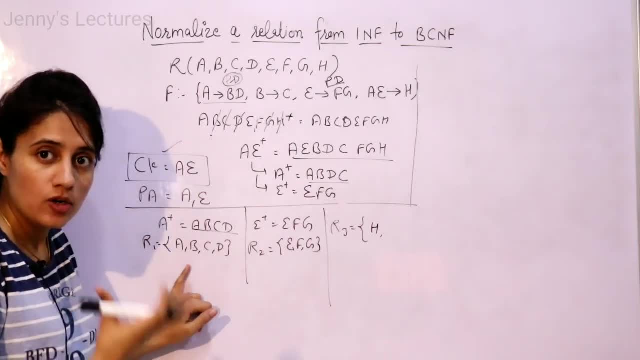 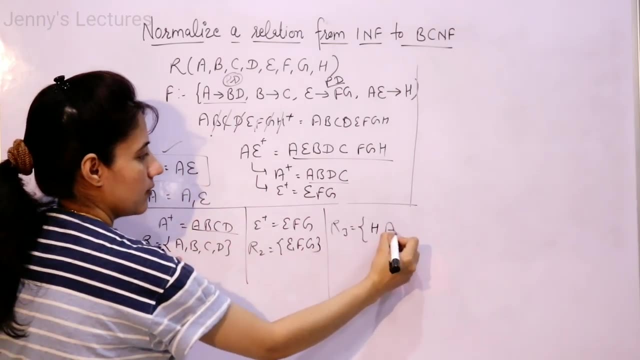 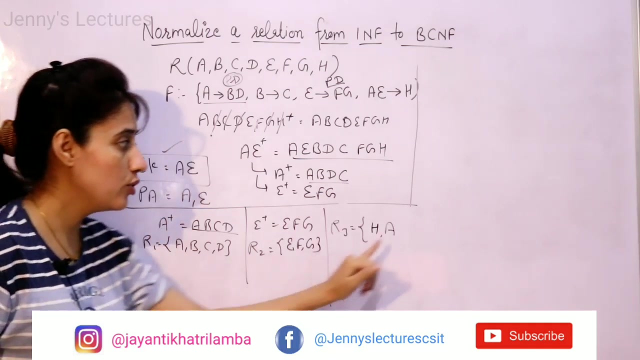 candidate key of at least one sub relation. right to be that decomposition and lossless joint decomposition, right. so suppose i put a common here. obviously a is candidate key for this one because because using a i can drive b, c, d, all the attributes, so it's better to put a common. you can put b common. 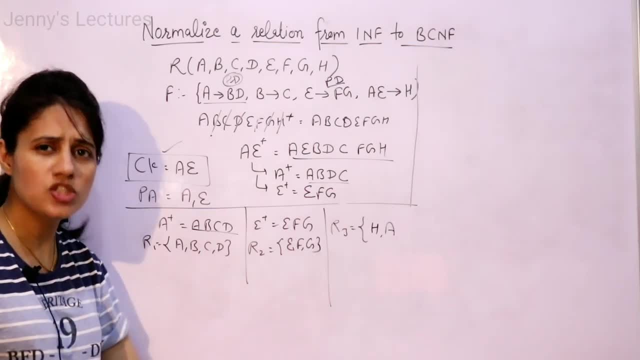 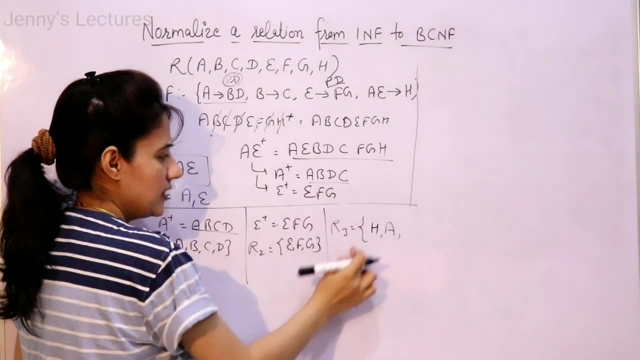 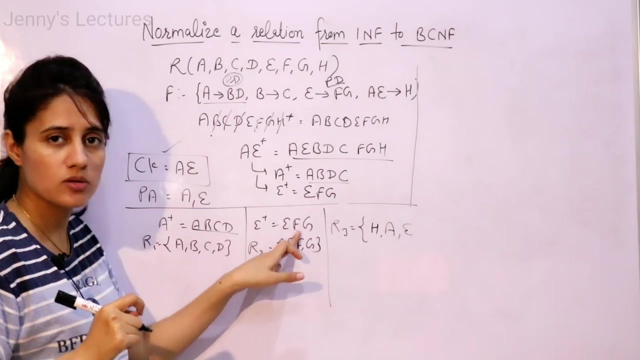 either c or d. you can put these things common and you can check out right. those would be loss c. joint decomposition right now between this and this, what should be the common attribute. it's better to put what e common because e is e is what candidate key for this sub relation, or you? 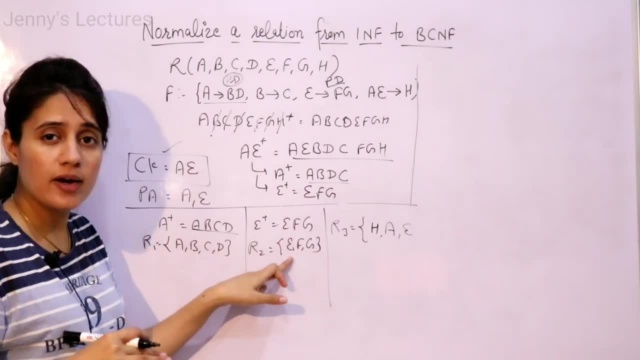 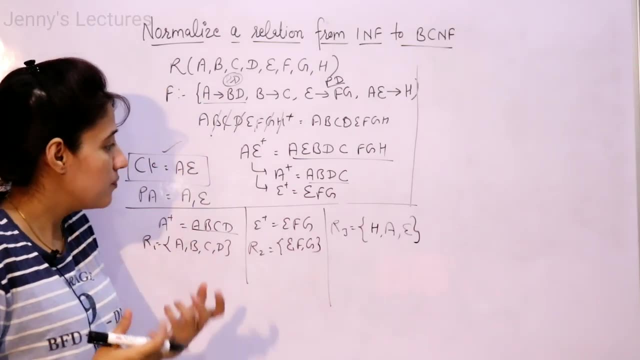 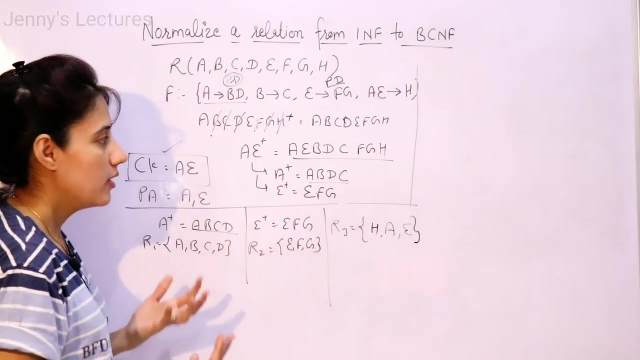 can say super key for the sub relation, because e can drive f and g, all the attribute of the sub relation right. so now this is a third relation or in simple terms you can say one. i mean in one relation we always put the candidate key, c. remaining attribute is h and 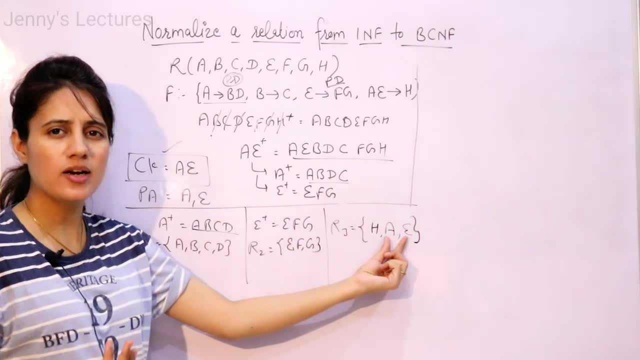 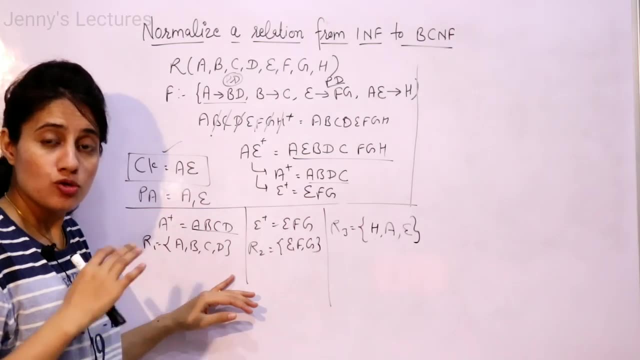 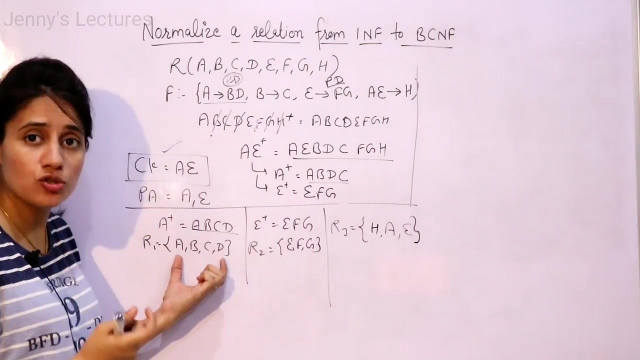 obviously the candidate key is what a, so we put a here, so that thing also you can consider or you can apply the the the logic which i am telling here in this video right. so now we need to check this- is lossless joint decomposition, right, but we need to check the, you know, highest normal form for this. 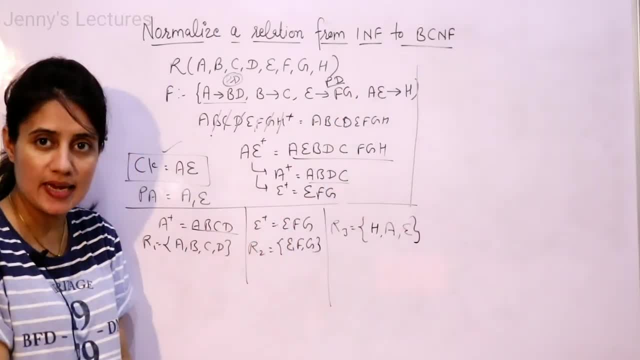 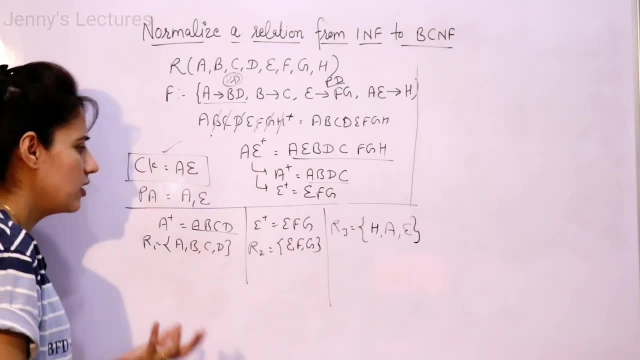 also. this also, and this also because we are supposed to convert it into b c n f right now. check it is converted into b c n f or not. or it is still in first n f or in second n f or third n f. we can't say so for that. we need to find out the functional dependencies. 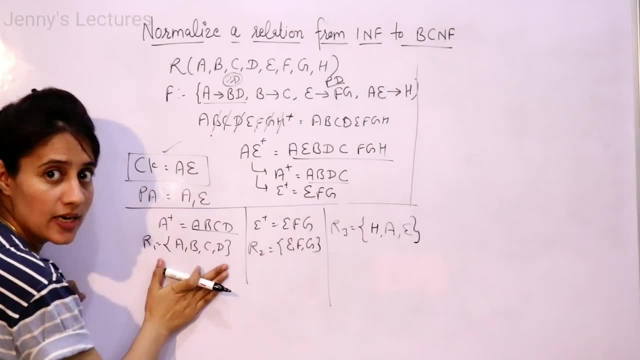 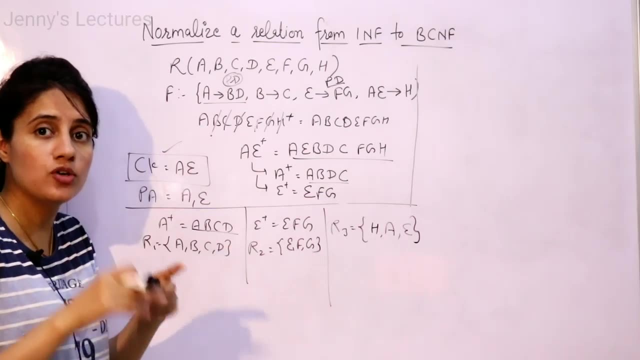 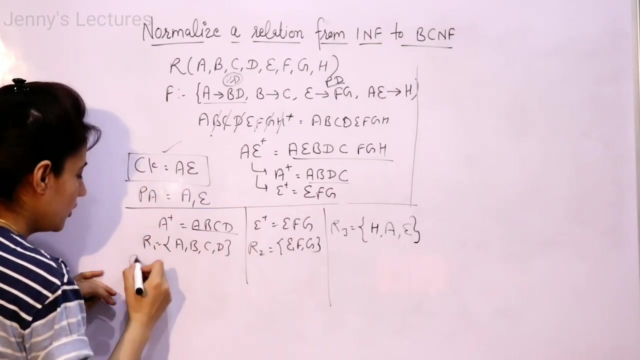 and candidate keys, right. so functional dependency for this relation would be how to find out functional dependencies. that video i have already discussed in detail. i will provide the link of that video, particularly in this i button. you can check out there here i am just writing the functional dependencies, right. so the functional dependency for this one. 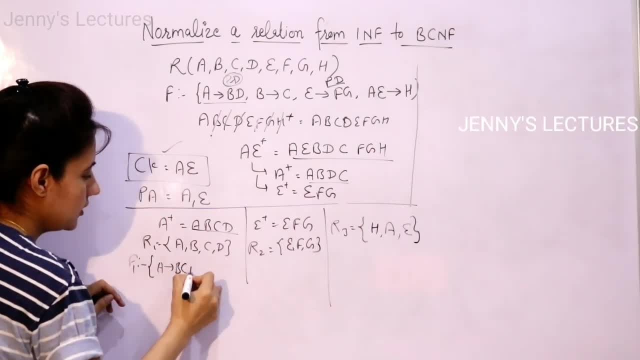 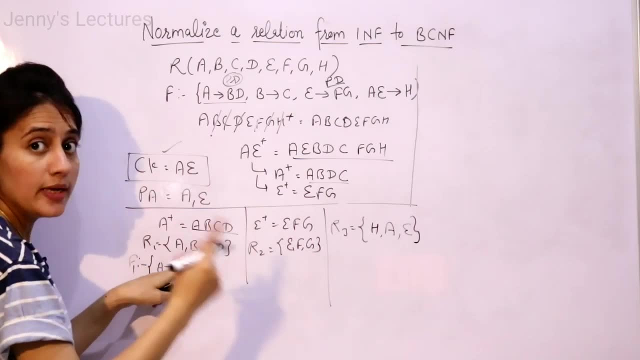 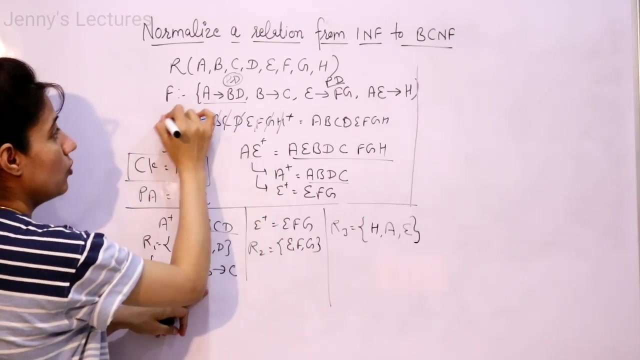 would be here. a can drive b, c, d, because when you find out a closer you will get this one and a to a is trivial and b, c, d right. when you will find out b closer, then you will get b to c- this functional dependency right. how to find out? you have to consider this functional dependency right now. if you find 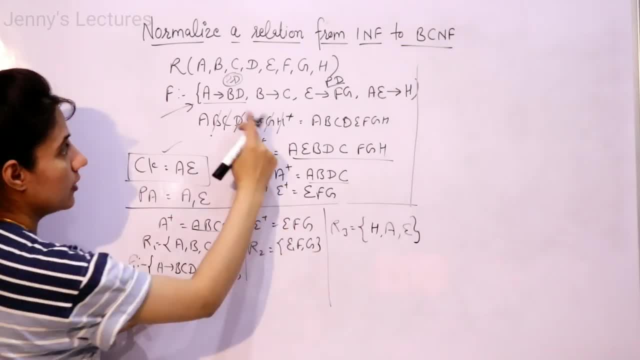 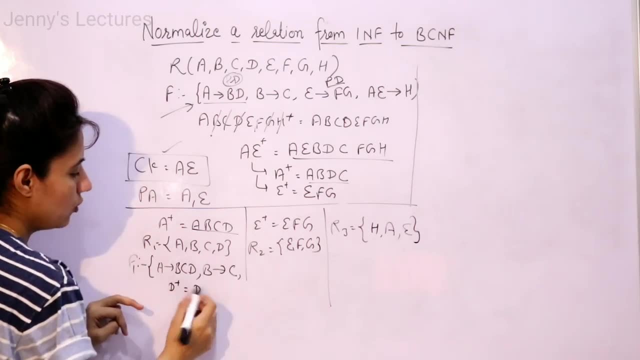 out c closer, then what would be the case? c closer would be c. only because c using c, i cannot drive anything. so this is trivial. so we are not going to take it d closer. also, we can only get d, nothing else. so this is also trivial, we are not going to take it right. 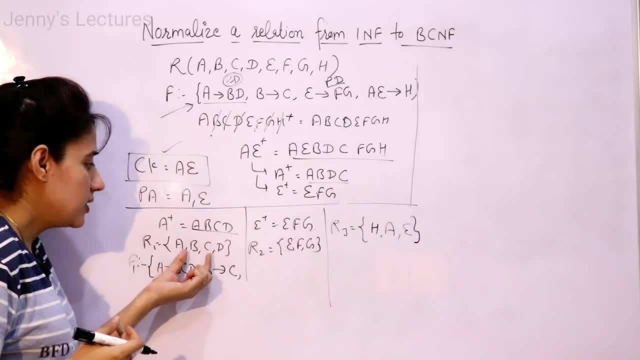 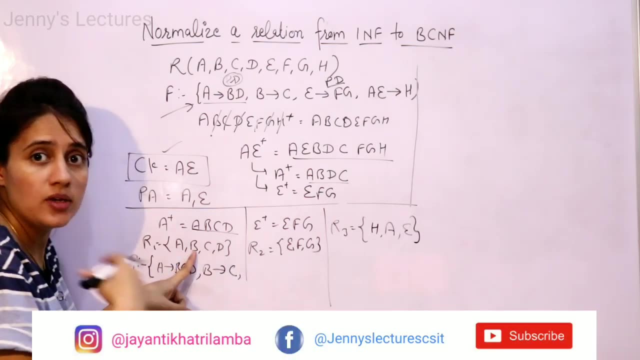 now a can drive all the attributes, so no need to check with a, b, a, c and a d like this, because that would be duplicate, right? and b can drive c, c and d are driving nothing, so no need to check b c, b d and c d, right? 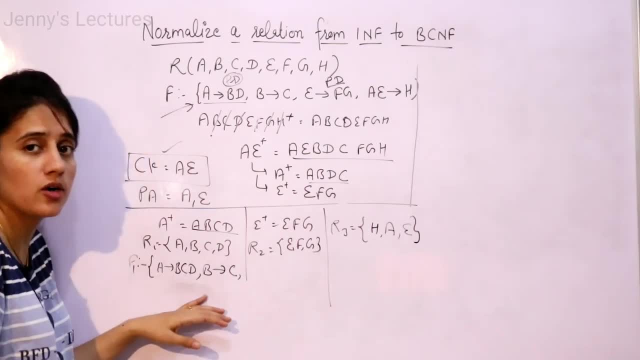 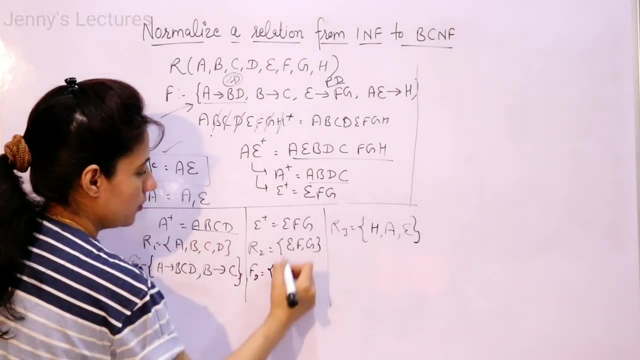 you will. you will not get anything. you will check, you can. if you want to check out, you can check out. right, so you will find out only these two functional dependencies here right now in r2, functional dependency would be: if you find out e closer, then f, g would be there. 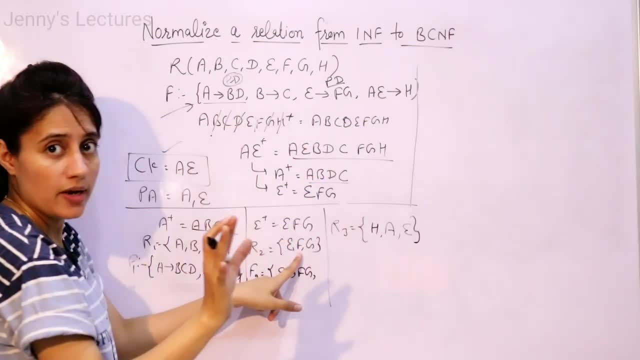 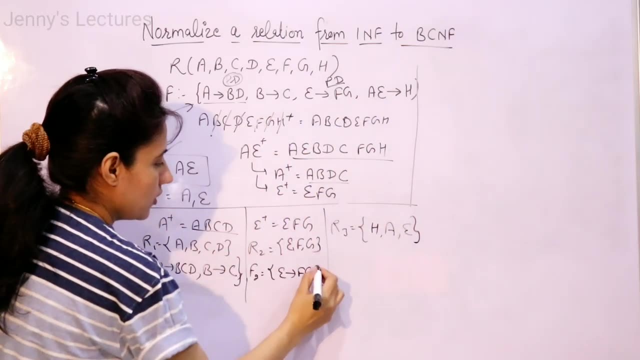 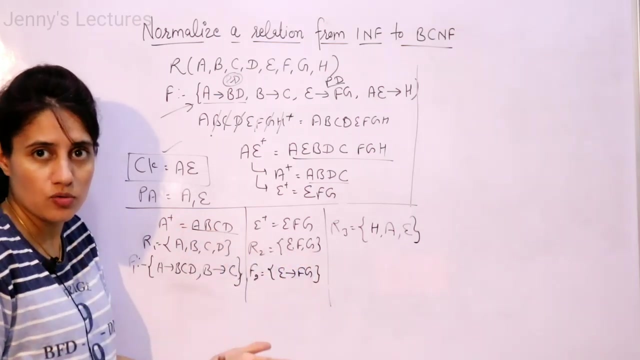 if you find out f closer, nothing you will get. f to f- trivial would be there- g closer, nothing will get using these functional dependency right. So there is only one functional dependency right. E can drive all the attributes, So no need to check E F closer and E G closer. 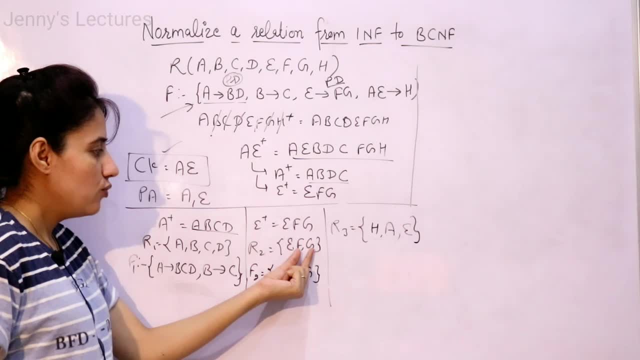 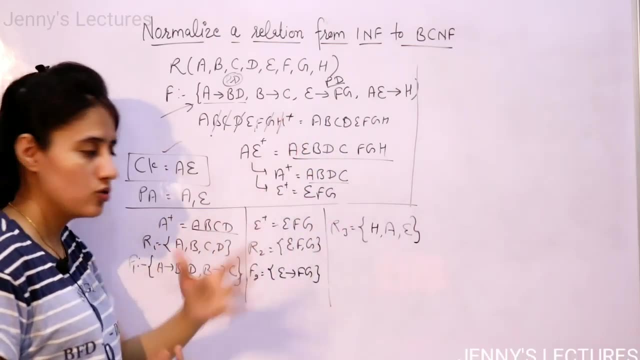 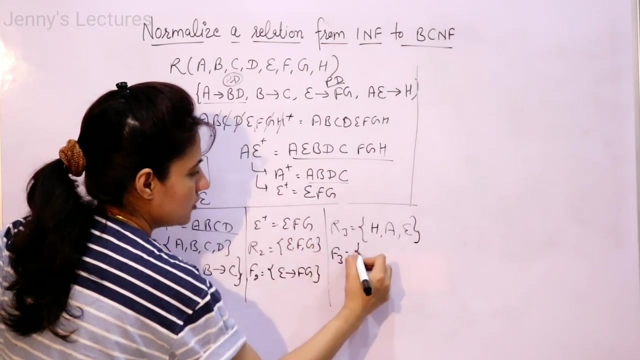 because obviously that would be duplicate and if you find out F G then that also would be trivial. only F G you can drive using F G. F G closer would be F G only right. So no need to take. there is only one functional dependency here. Now, here functional dependency. 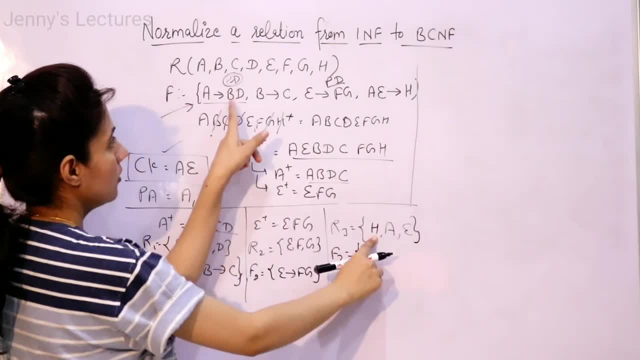 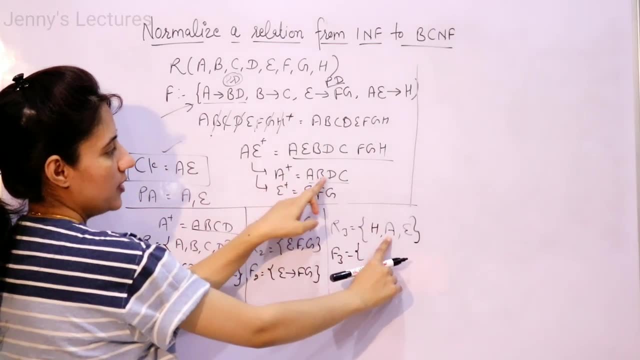 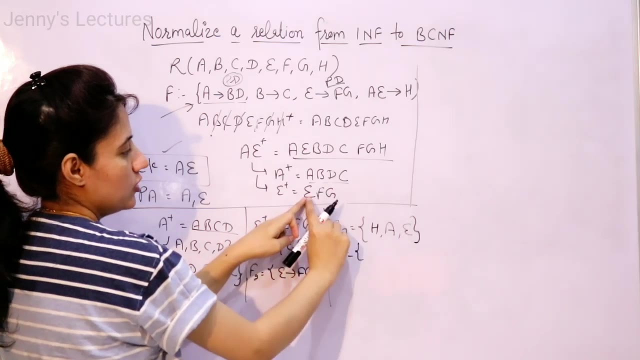 would be see, if you find out H closer, you will get only H trivial. If you find out A closer, then you will get this one. but A to A is trivial. B, C, B, C, D are not part of this one, So no need to take this one. we are not going to take E. closer would be E, F, G, E to. 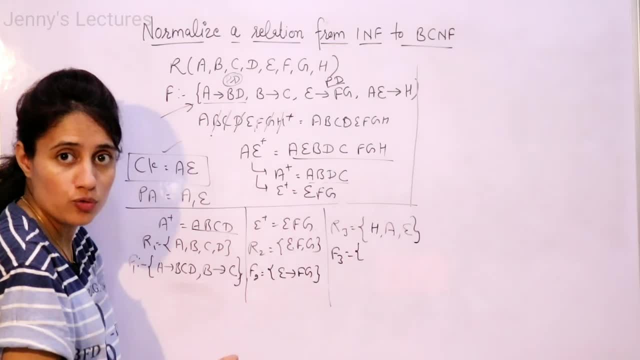 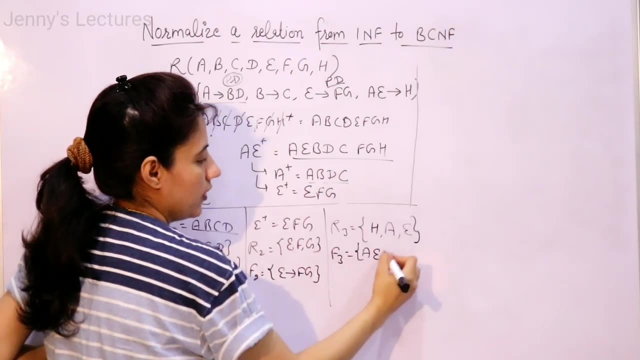 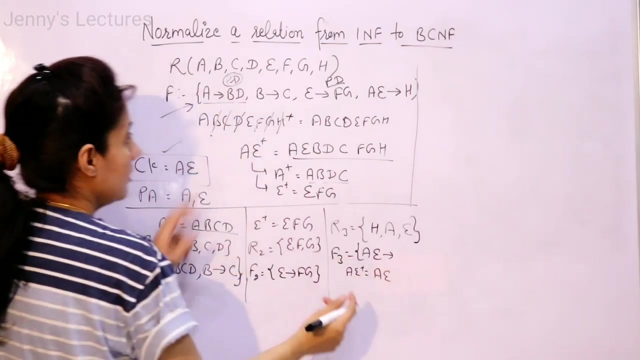 E is trivial. F, G is not part of this sub relation, So we are not going to take it right. So now, one relation, one dependency would be there here: A E. If you find out A E closer, then that would be A- E. using A, I can drive, B D. using B, I can drive, C. using E, I can drive. 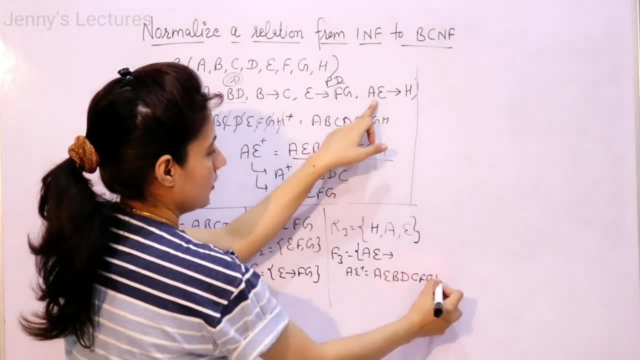 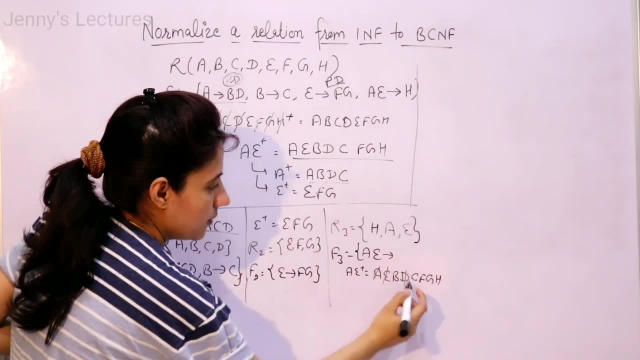 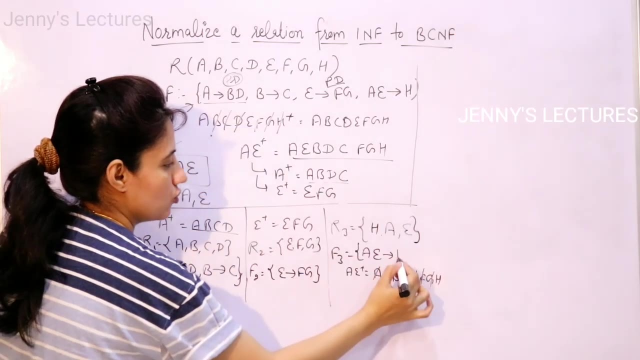 F and G right. using A E I can drive H. all the attributes A E to A E is trivial, see. D is not part of this sub relation, C is not part of this sub relation. F is no and G only. H is part of this sub relation. 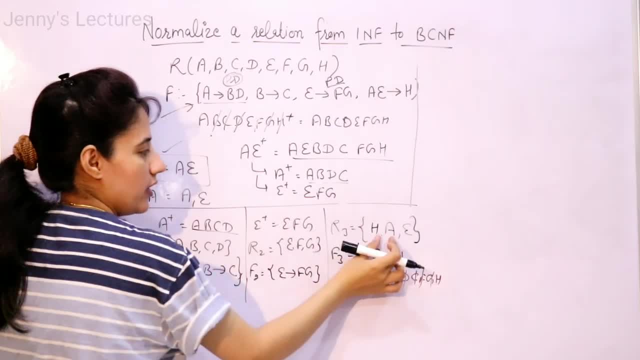 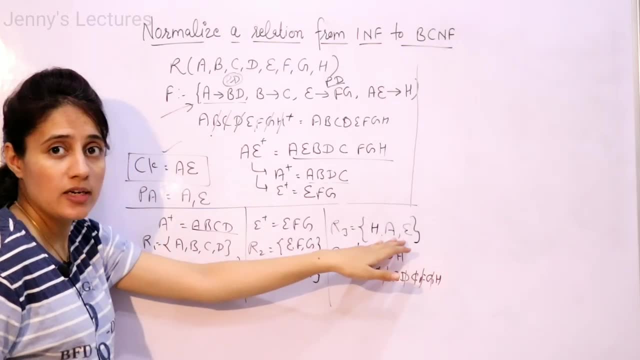 so A, you can drive, H, right, same you can find out A, H, same you can find out E, H, right. you will get nothing. all the attributes, those you will get in closer, that are not part of the sub relation, right. so we are not going to take those functional dependencies. so 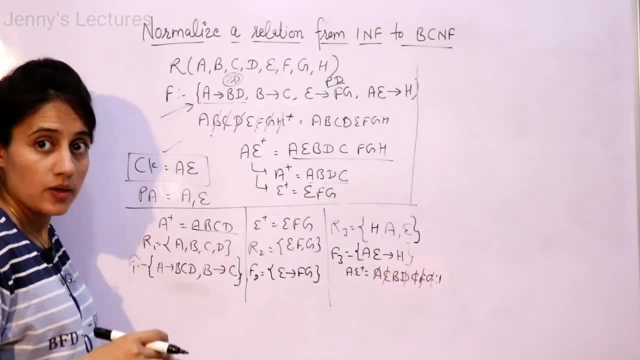 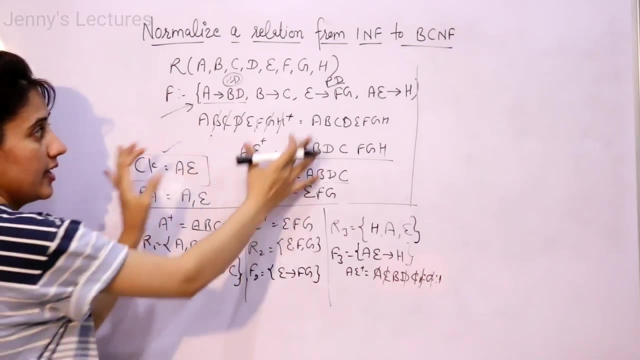 only one functional dependency would be there in this case. right now, find out the normal form for this, this and this same. for that you have to find out candidate key. the same process you will apply in each sub relations. right, I am not going to apply again because 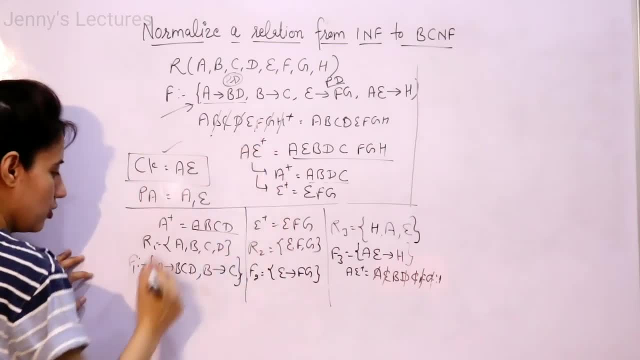 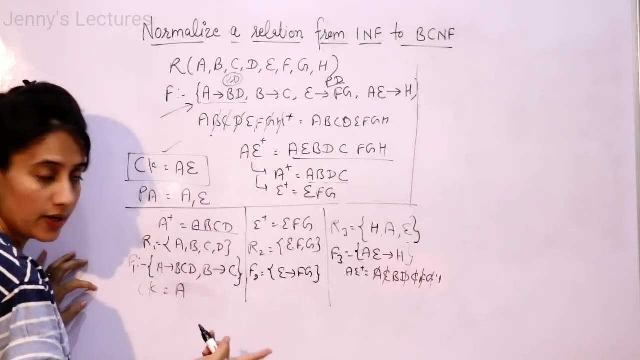 we have already discussed one time. so when you apply the same process then the candidate key for the sub relation would be A. from here only you can check A can drive all the attributes right. so candidate key would be one. candidate key is A and A is not on. 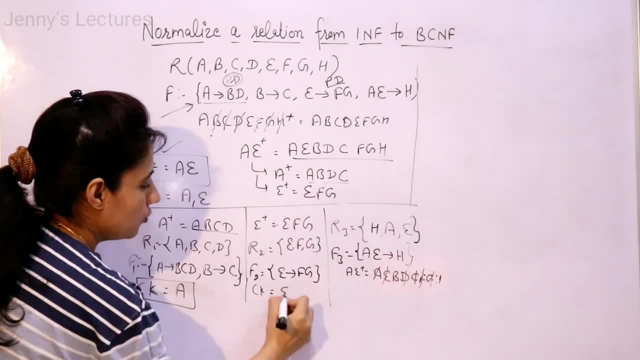 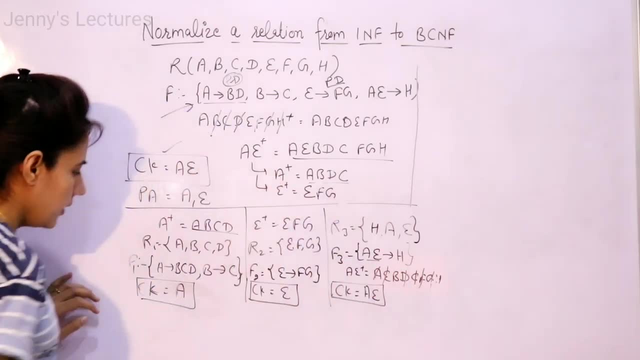 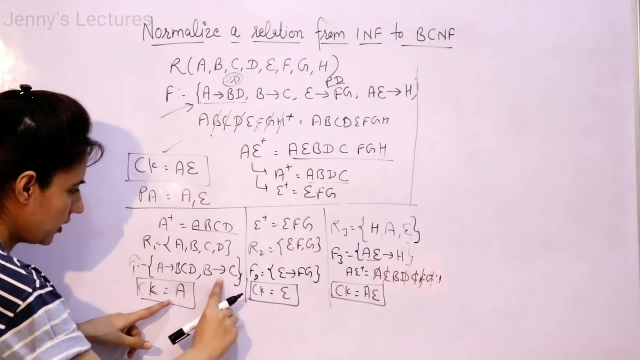 the right hand side. so there is only one candidate key. here the candidate key would be only E, and here the candidate key would be A E. Now see, is this partial dependency? no, is this partial dependency? no means this. 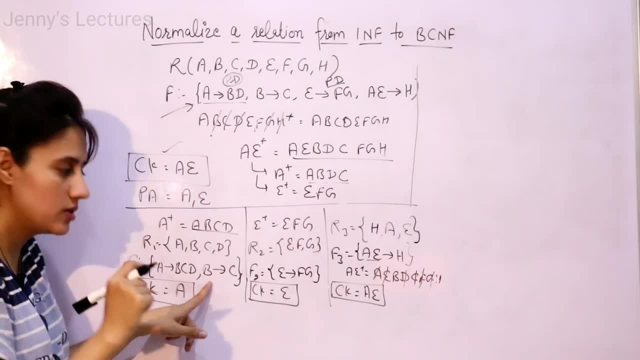 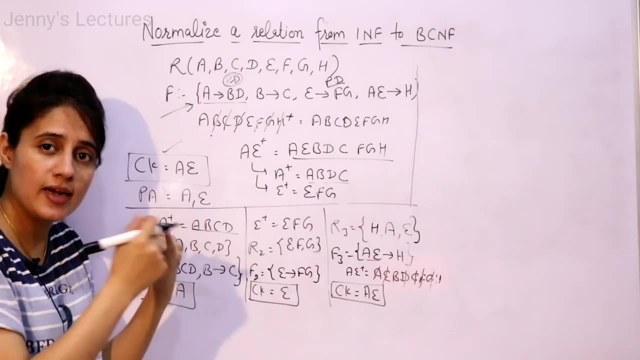 is in second NF? definitely, but is it in third NF? see check for three NF. two conditions are there. one of those two conditions should be satisfied. either left hand side is super key or right hand side is prime attribute. is left hand side super key? yes, so this. 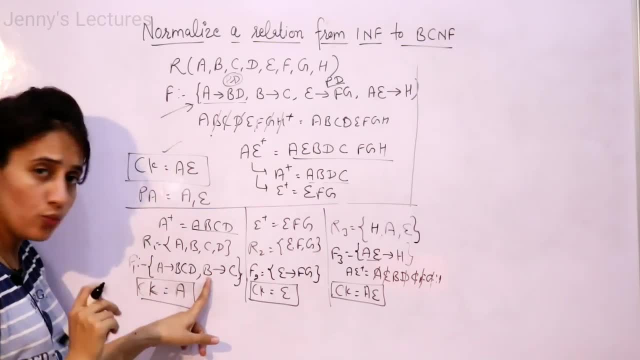 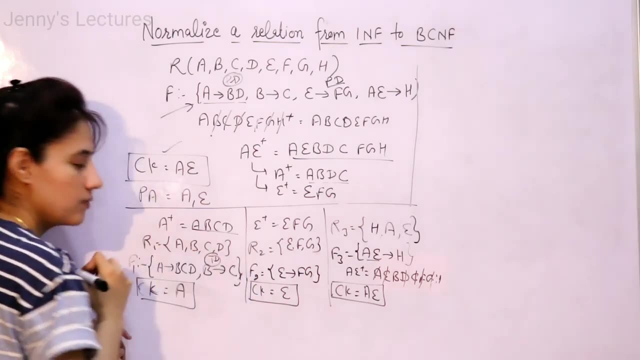 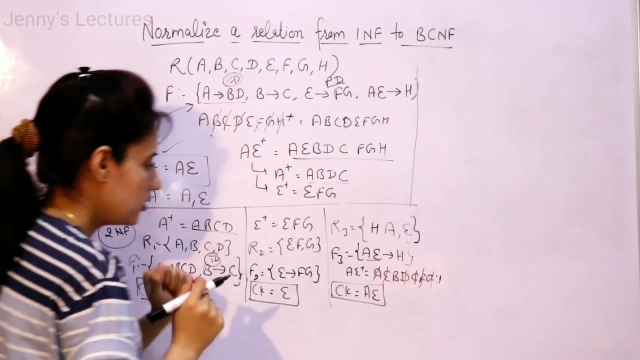 is not transitive dependency. right Is left hand side super key. no, is right hand side prime attribute? no, because prime attribute is only one A. so this is transitive dependency. so this relation is not in third normal form, it is in second normal form. R1, check for this. one E: the left hand side. 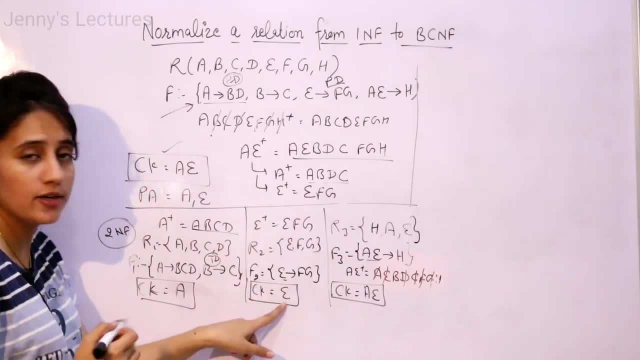 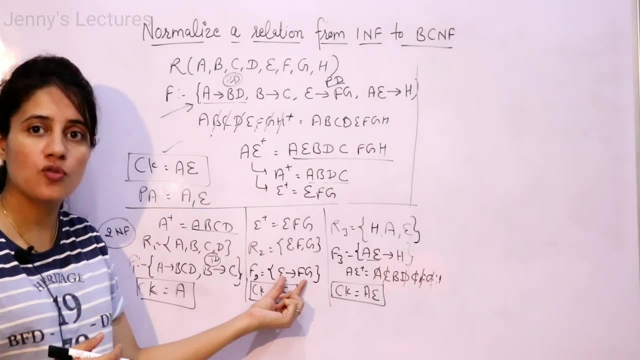 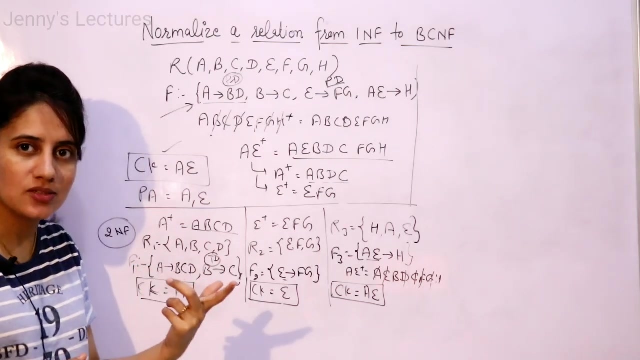 is what only one dependency is there and the E is what candidate key or you can say super key, right? so if the left hand side is super key of the functional dependencies, of all the functional dependencies, Then that relation is in BCNF, that rule we already discussed, right? so this is in. 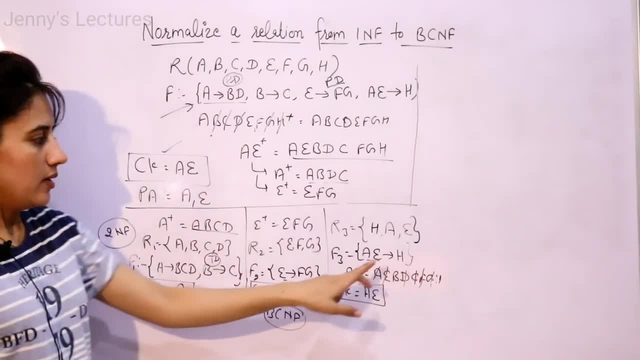 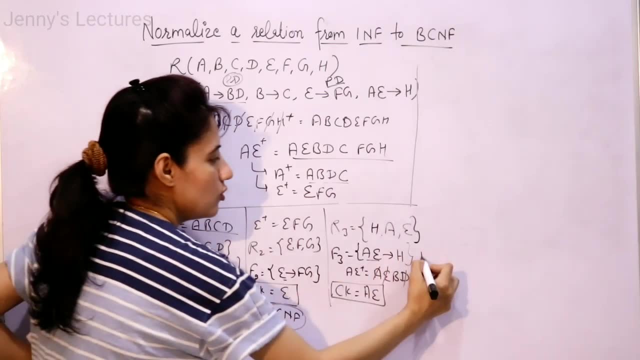 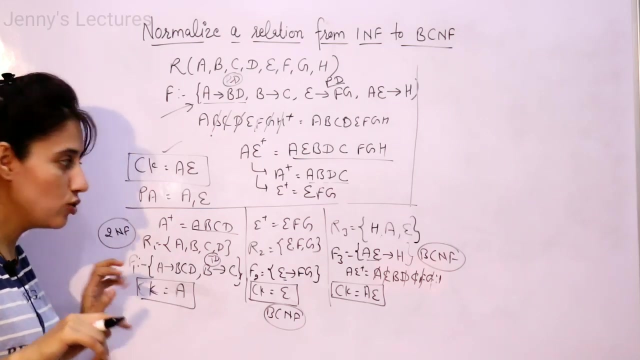 BCNF- this one left hand side- is what super key, or you can say candidate. obviously candidate key is super key also, right? so this is also in BCNF. but this is in second NF, right? so it is not like that we have got two BCNF. so it is in BCNF now. no, it is still in second. 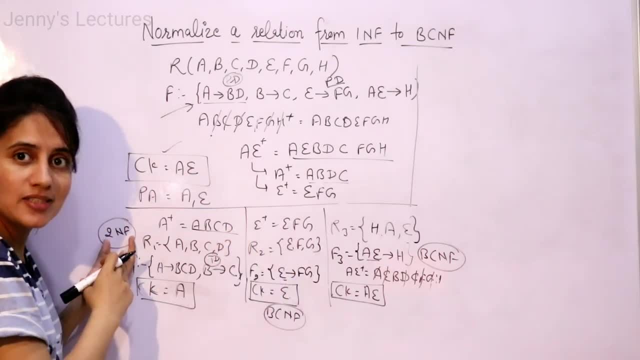 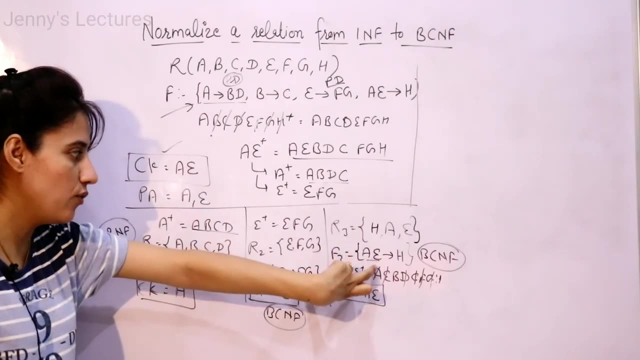 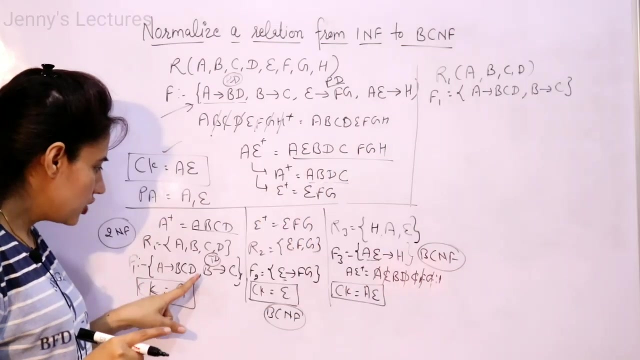 normal form because the lowest one we are going to choose. right, that is second normal form. now you have to convert this sub relation only into third NF or BCNF. this we have already got two sub relations. right now we are going to work on this R1 only now here, which functional. 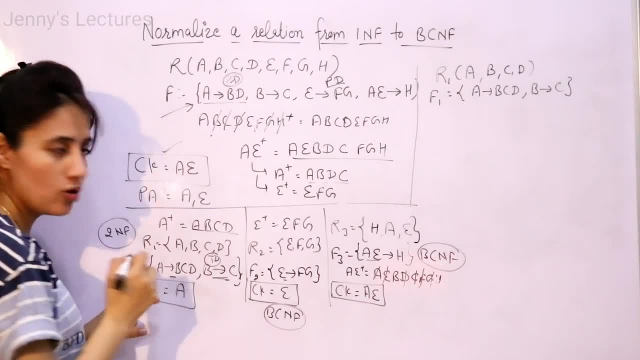 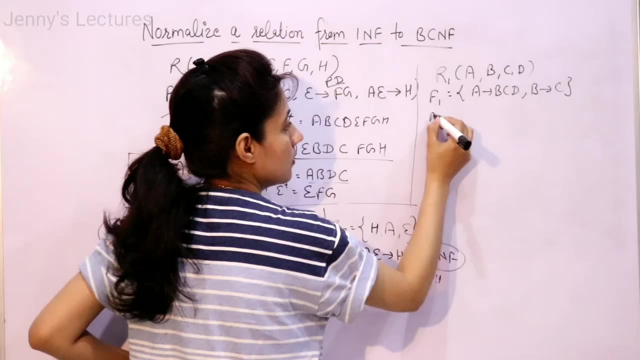 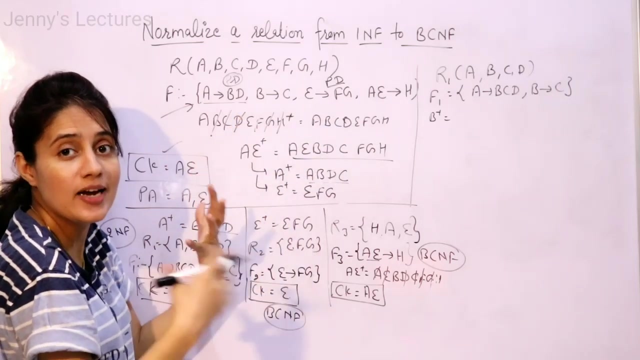 dependency is creating a problem. for third NF, this one only because this is not creating a problem. this is not transitive dependency, this is transitive dependency. so now take B closer. Samantabhad Kalani. Now see, we are not going to consider now this functional dependency, because now we 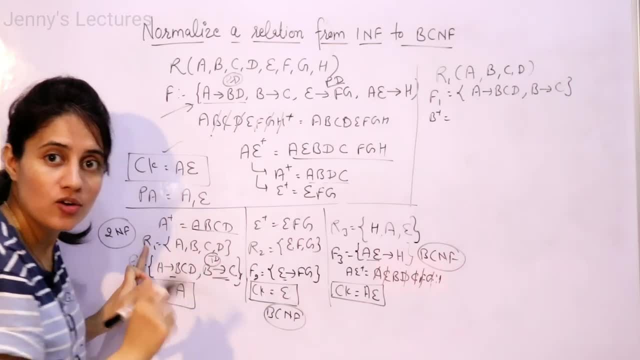 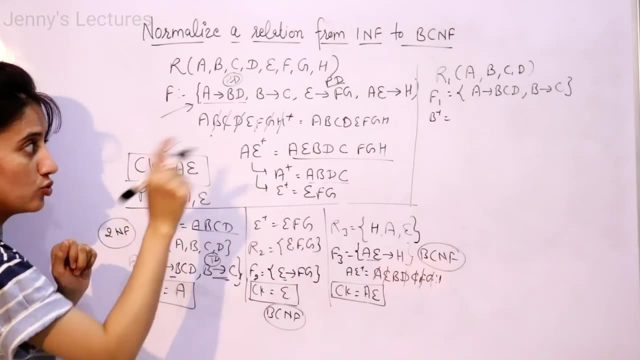 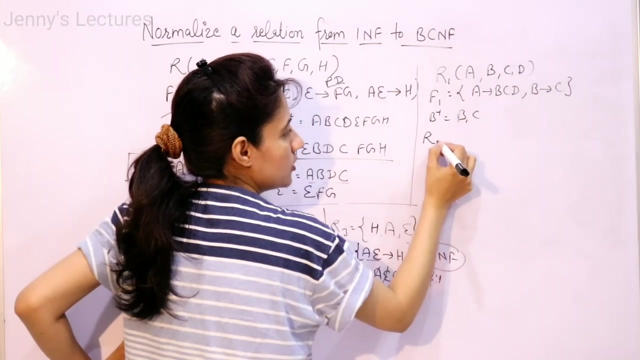 are decomposing this relation R1, and we have already got this functional dependency set for this sub relation. so now we will consider this one to find out B closer, so B closer would be B, and using B I can derive C, only BC, so one sub relation would be, suppose, R11. 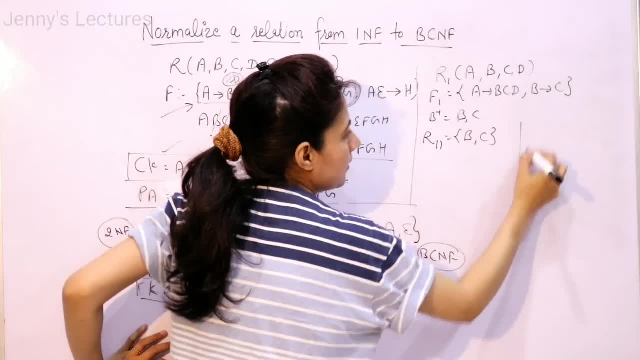 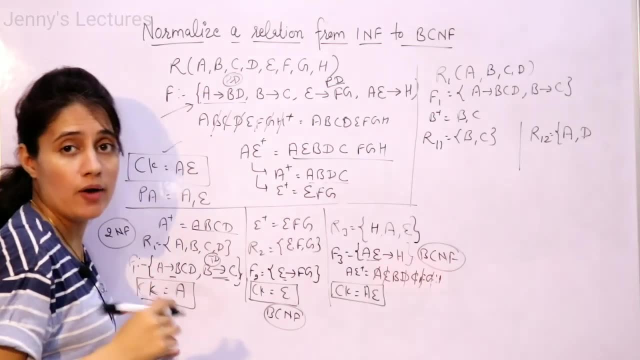 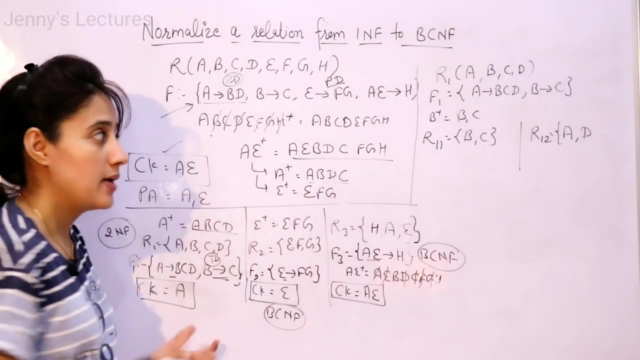 that is BC Samantabhad Kalani. meaning would be in second sub relation, that is a and b. now we have to put something common right to get a lossless joint decomposition. common should be at least super key of one sub relation. as we know, b can drive c, so b would be definitely super key. or you can say candidate k for this. 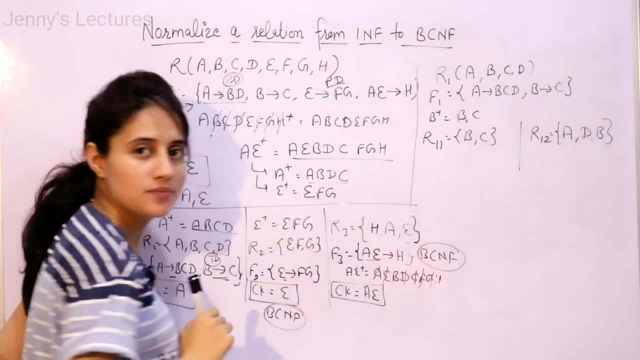 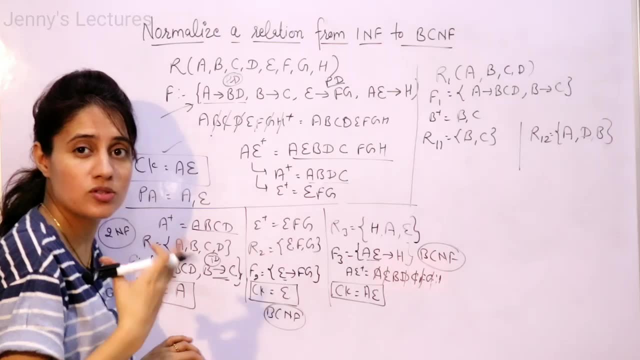 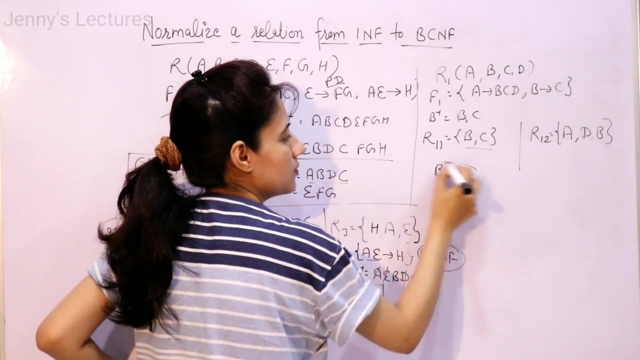 sub relation. so better to put b common right now. find out functional dependencies and then find out that this is: or this is in b c n f or not, or still in third n f or still in second n f. this is having only two attributes, so this is definitely in b c n f right. check for this one, find out. 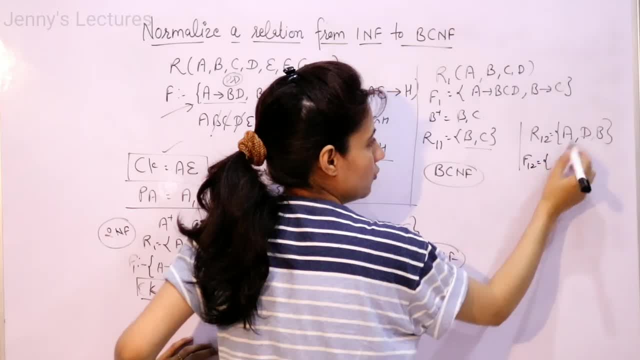 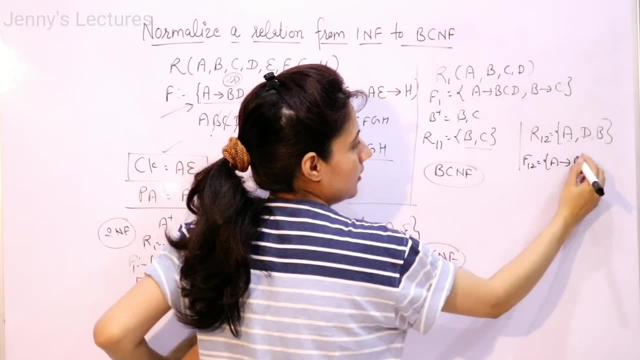 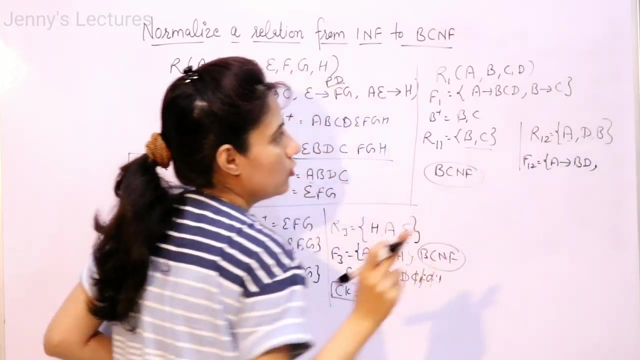 functional dependencies. first, f 1, 2 set would be: if you find out a closer, you will get a can drive b c. d means b d because c is not part of the sub relation, right? if you find out d closer, nothing you will get. trivial functional dependence you will get if: 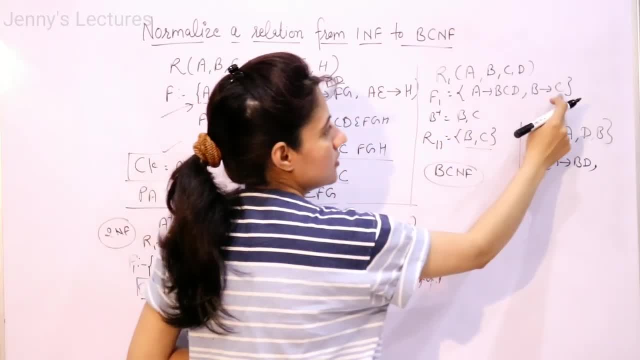 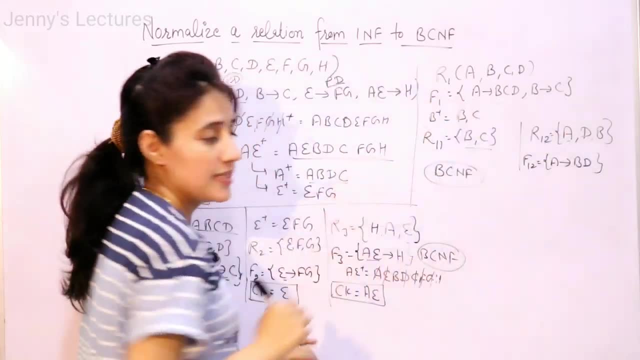 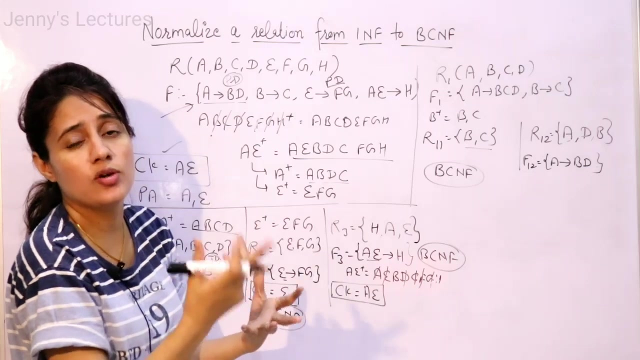 you find out b closer, then you will get b and c. b to b is trivial and c is not part of the sub relation, so we are going to take only this one right because a can drive all the attributes, so no need to check a, d and a b closer right. and if you want to check b- d closer, then you will get. 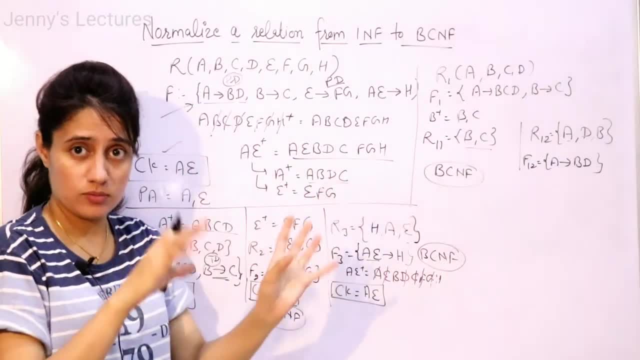 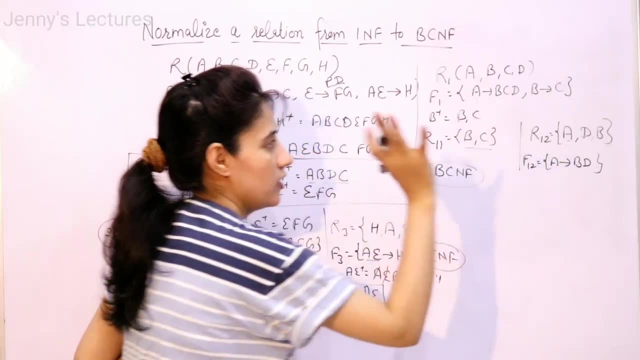 what b, d and c only. so b, d is trivial, c is not part of this one. so you will get b to b and c one. so we are not going to take that functional dependency also right. so there is only one functional dependency. now if you find out the candidate key, then candidate key would you will. 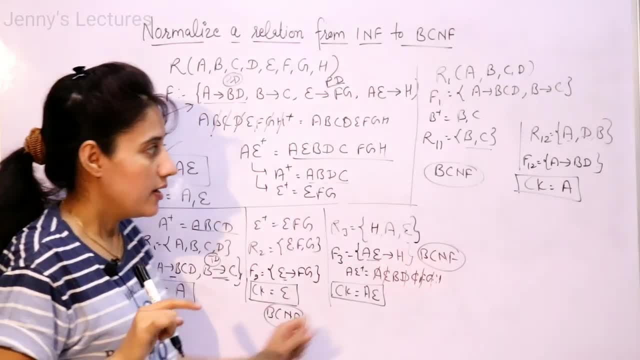 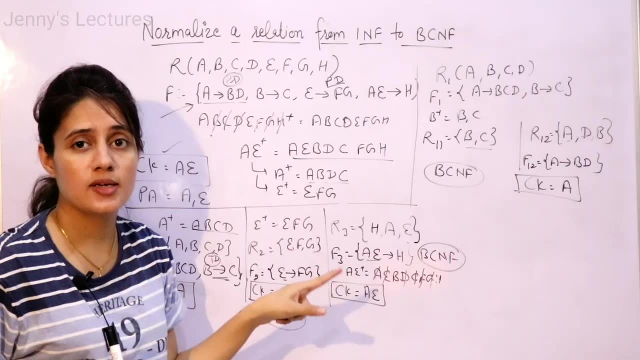 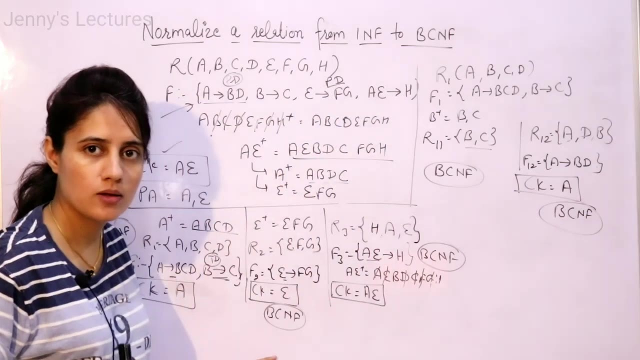 get. that would be a only right now. if you check left hand side of this, functional dependency is a, that is candidate key or you can say super key. so this is definitely in b c n f. so now this is in b c n f right now. ultimately, finally, we have converted it into a functional dependency. 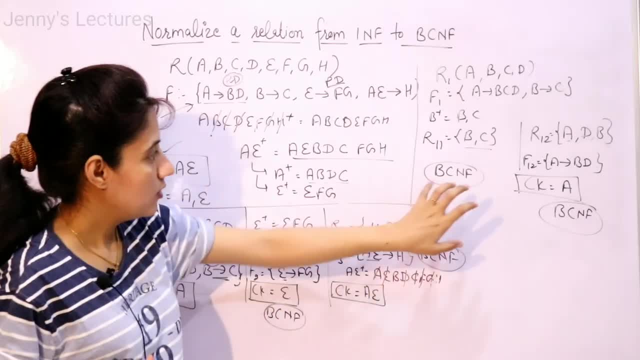 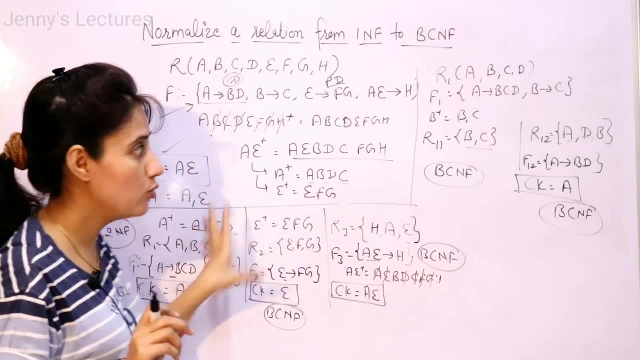 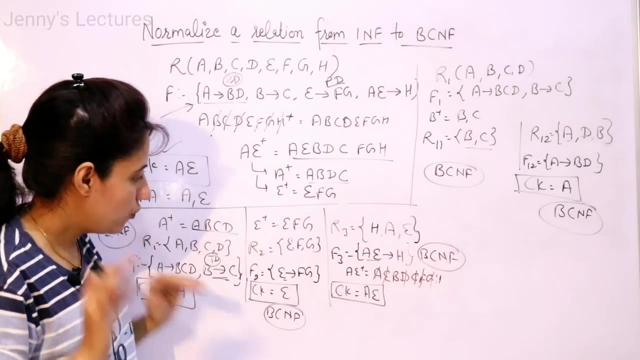 into b, c, n f right, because. and now, how many sub relations are there? one, two, three and four. we are not going to consider this because we have decomposed it into this one to to convert it into b, c, n f, because it was in second nf right. so four sub relations are there: this one, this one, this one. 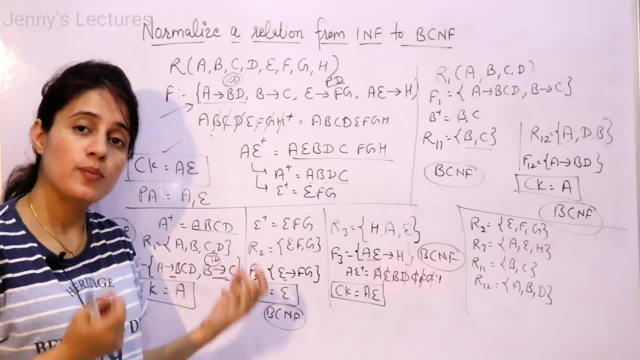 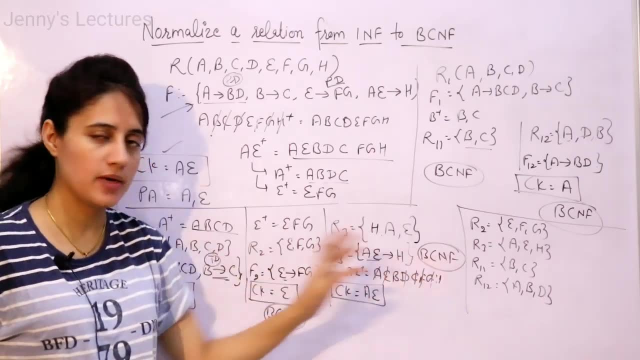 and this one. and if you are asked how many sub relations would be required to convert this into b, c, n, f, then your answer would be four sub relations would be required. these four sub relations, right? this is how. this is the step-by-step explanation, how we are going to. 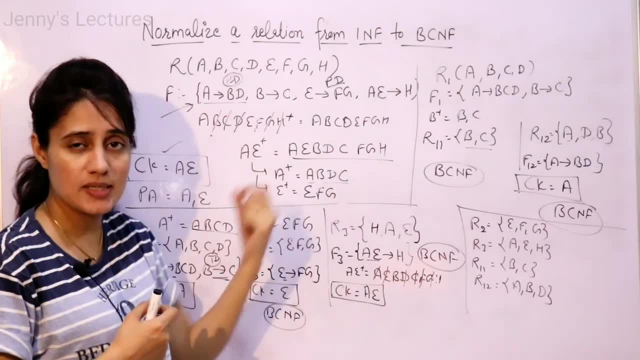 convert a relation which is in first nf to first nf to b, c, nf. right, so that's it for today. now i'll see you in the next video. till then, bye, bye, take care.